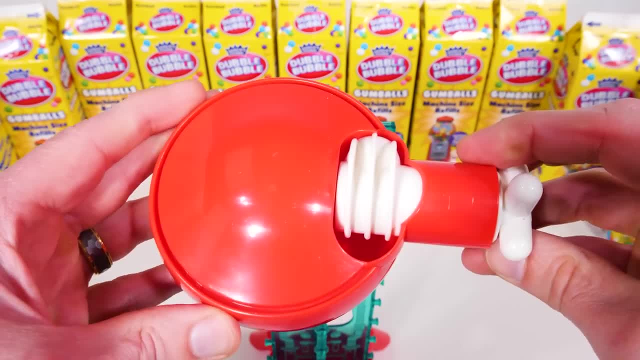 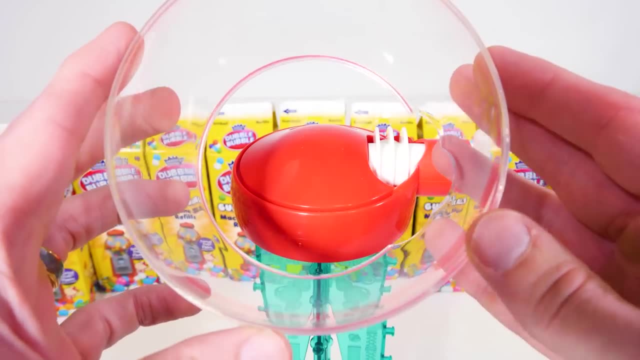 this little scooper which will grab the gumballs and send them out through the hole here at the bottom, And this little piece is going to go right here Now. on top of this we'll assemble our globe- Here's the bottom half or bottom hemisphere of our globe- and it'll go on the dispenser. 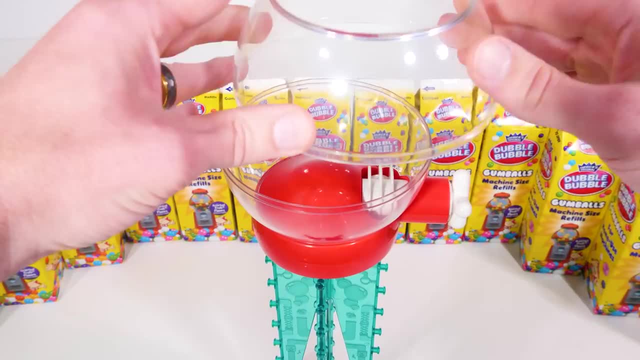 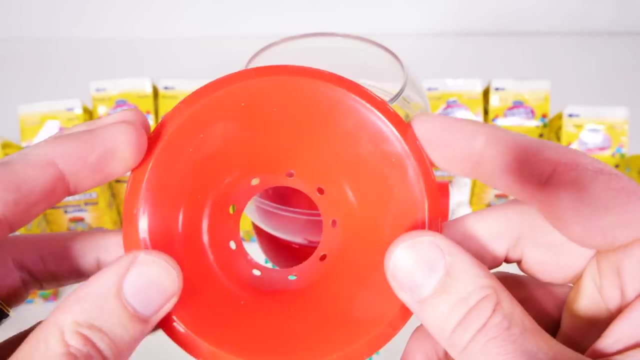 And now the top half or top hemisphere, And of course that's going to go on the top. Now it's looking like a real gumball machine. We'll just need to add this funnel that'll guide the gumballs into the globe. 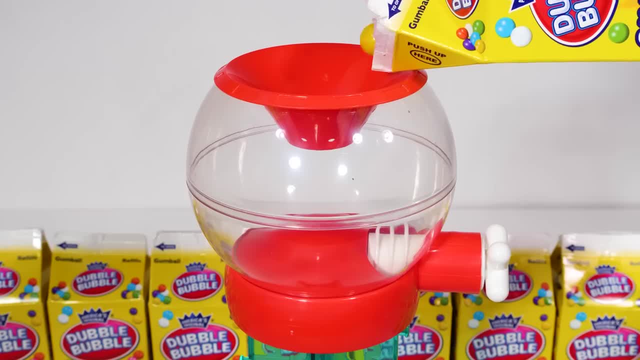 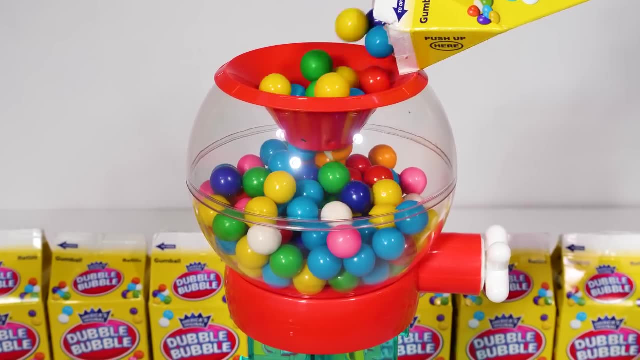 And now for the best part, adding the gumballs to the gumball machine. I think we should try to fill it up all the way They're getting there. Oh no, we clogged the funnel with gumballs. Looks like we'll need to move it if we're. 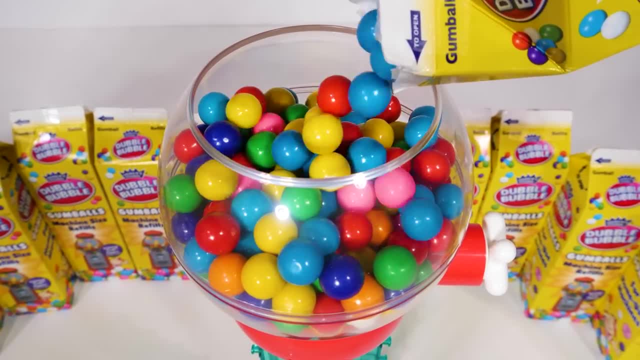 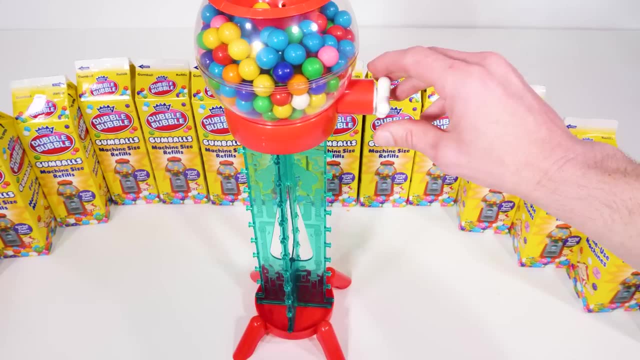 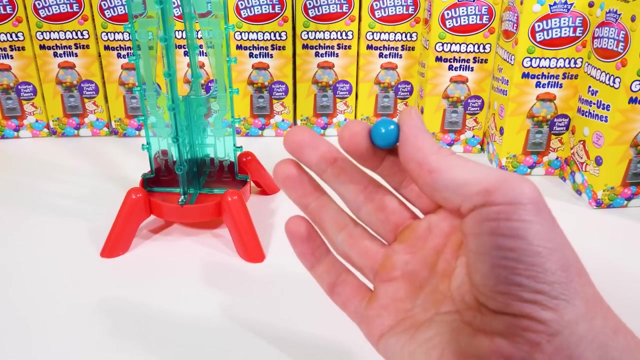 going to fill it up all the way. All right, that's looking a lot better. Now, if we turn the handle of the gumball machine, gravity will pull the gumball down to earth. Now we all know about gravity, but did you know that all things have gravity, Even this gumball? 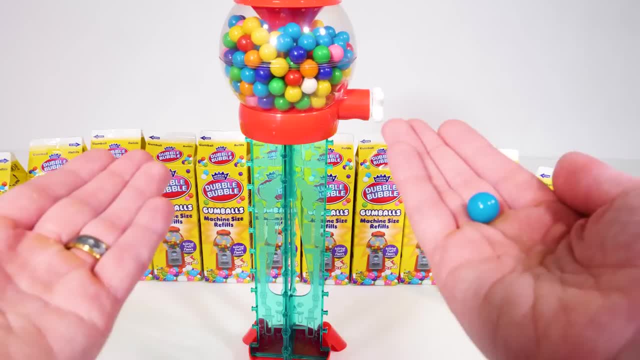 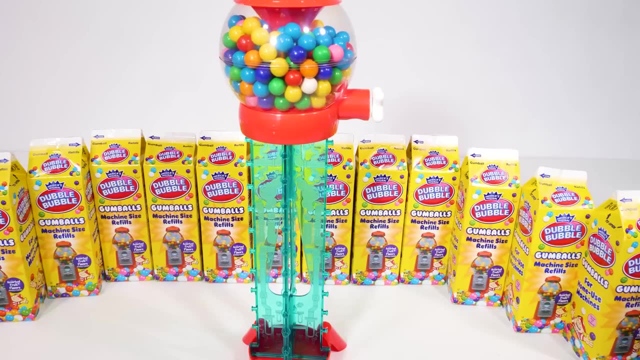 Even you. It's just too little to notice. But using just gravity on our gumball machine is boring, So let's try to add some other forces to see if we can have a lot more fun. The first thing we can use is a little trampoline. Its bouncy springs will collect the falling. 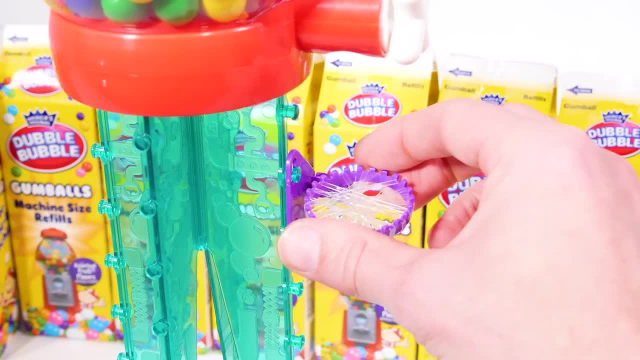 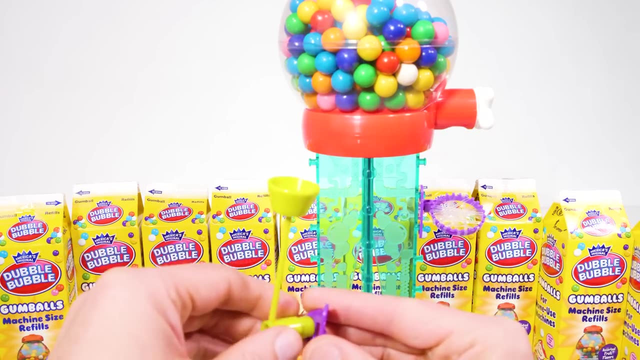 gravity energy of the gumball and then shoot it back up against the force of gravity. We just need to attach it and aim it just a bit. Next we'll use this pendulum And you can see that it returns to the same state. 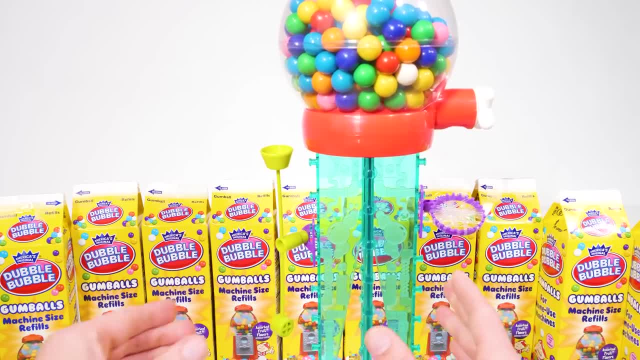 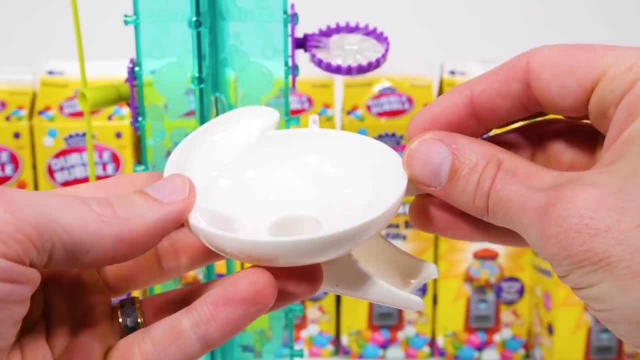 even after we knock it. That's because pendulums are stable. Using this funnel, we'll get to see some centripetal force as the gumball moves around in a circular motion, And if you want to experience it yourself, just ask your parents to spin you around by the arms. 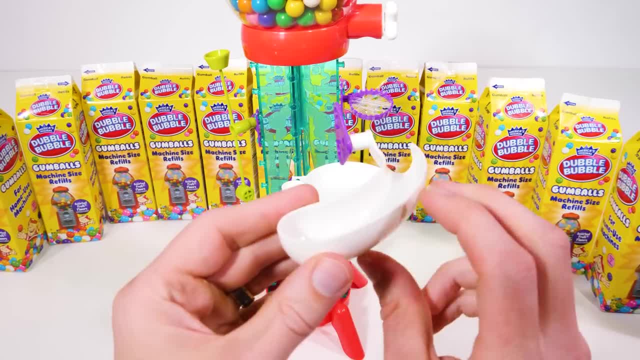 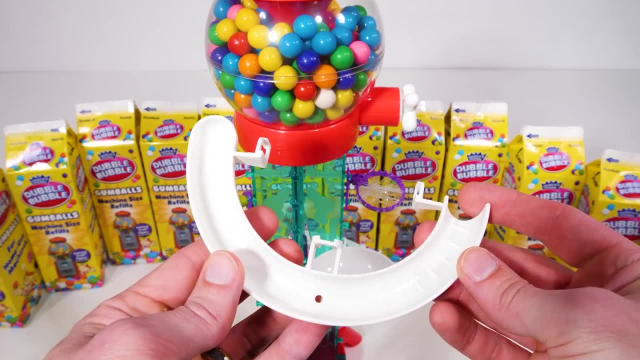 Next, we'll use this declining plane or a ramp to guide the gumball down the track And it just snaps on like the other pieces did. There we go, And here's a ramp to play with the speed of the gumballs. 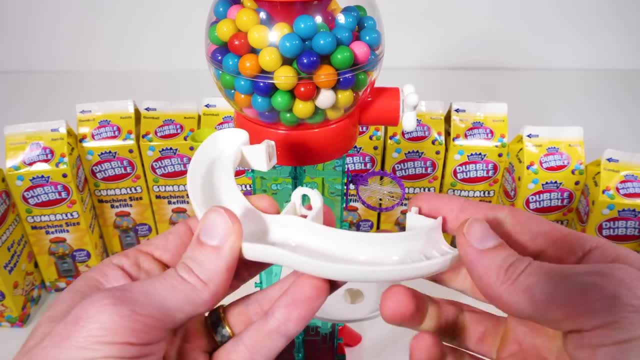 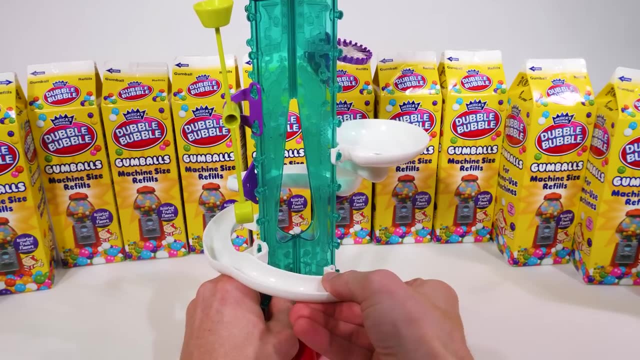 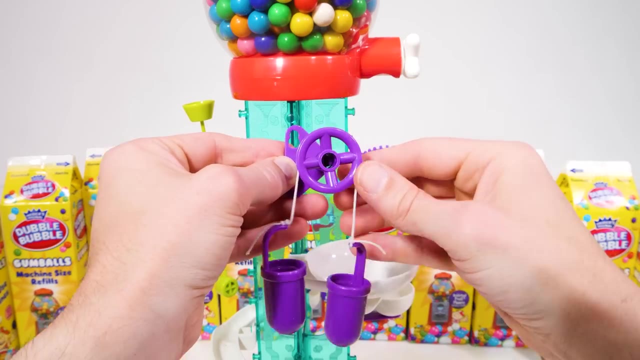 It has little bumps on it that cause friction. that'll slow it down as it rolls across it. Did you know that friction can even cause heat? Try it. Rub your hands together and see if they feel warm afterwards. And the last thing we're going to add is a pulley, which is a mechanism that uses a wheel and a rope. 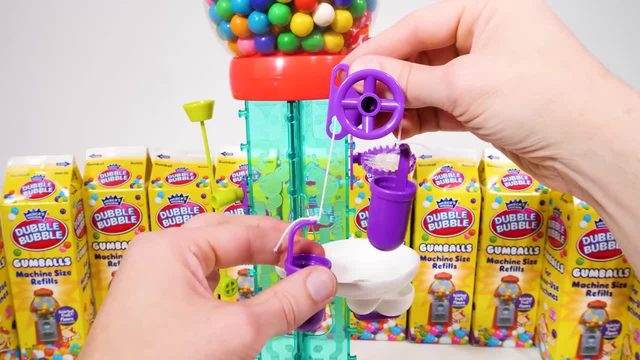 to change directions of force. If we pull one side down, the other one goes up. Pulleys have been around for thousands of years and have helped to keep the gumball from falling. So let's try it. Pulleys have been around for thousands of years and have helped to keep the gumball from falling. So let's try it. Pulleys have been around for thousands of years and have helped to keep the gumball from falling. So let's try it. Pulleys have been around for thousands of years and have helped people build tons of cool stuff throughout history. 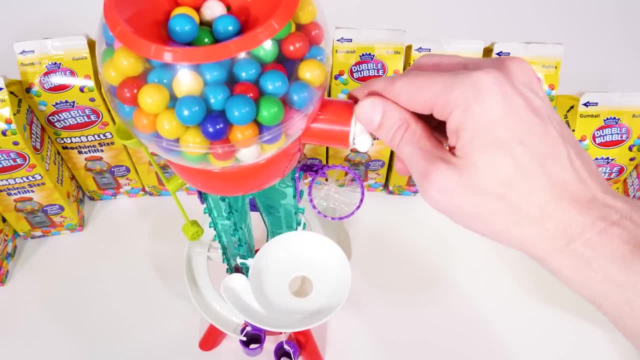 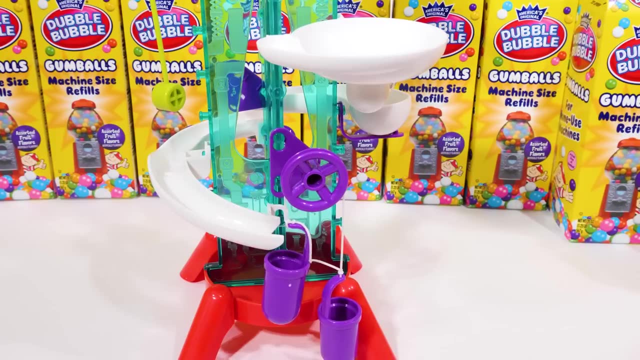 Alright, guys, what do you say? we try out our gumball machine. I wonder what color we're going to get. Oh, a red one. Look, the centripetal force is spinning the gumball And down the track. 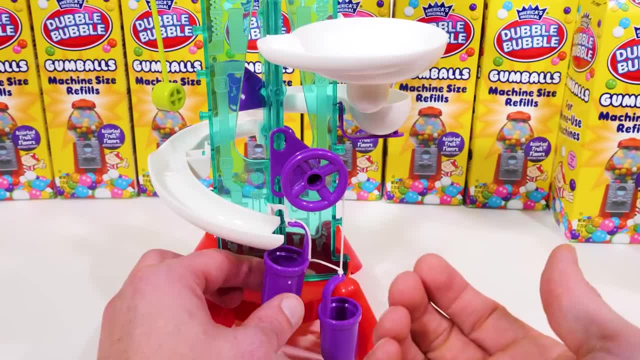 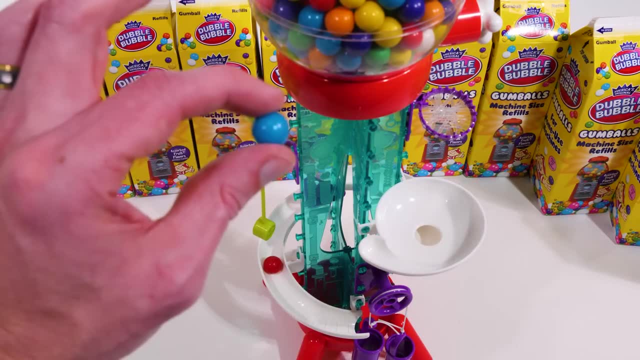 into the pulley. Wow, awesome. Now let's get our red gumball back and we'll try something new with it. Let's stick it over here on this part of the track, Then we can use a blue gumball, with the help of the pendulum, to knock it in. Thank you, pendulum. 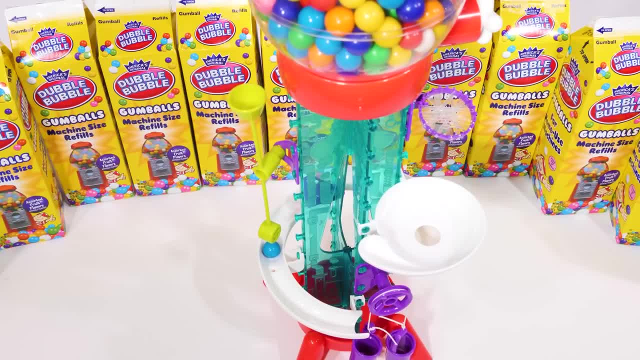 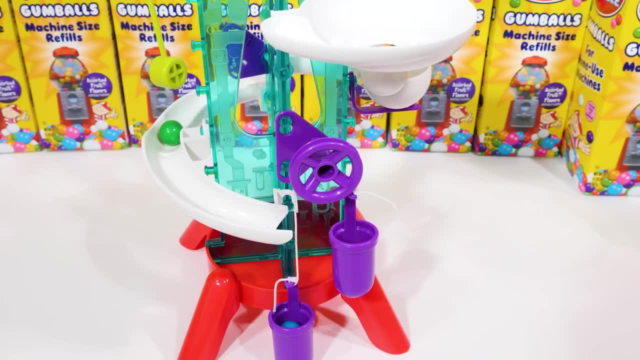 Oh, here it comes Alright, right into the pulley. Alright, let's give it another try. Whoa, a green one. Wow, that time the pulley really worked. That was so cool. Now let's try another configuration. 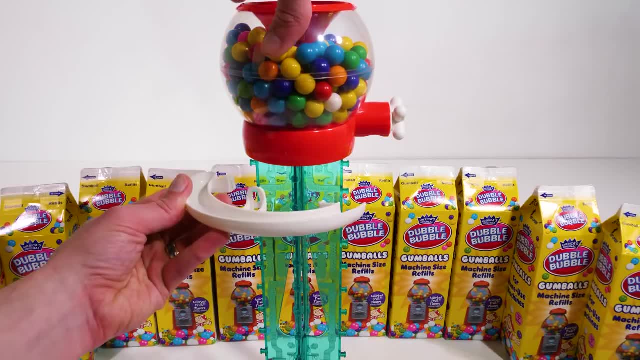 Alright, for this build, we're going to start with a C-shaped turn piece And we're going to hook it right here, so it ends just under the dispenser, And next to that one, we're going to put our friction track over here. 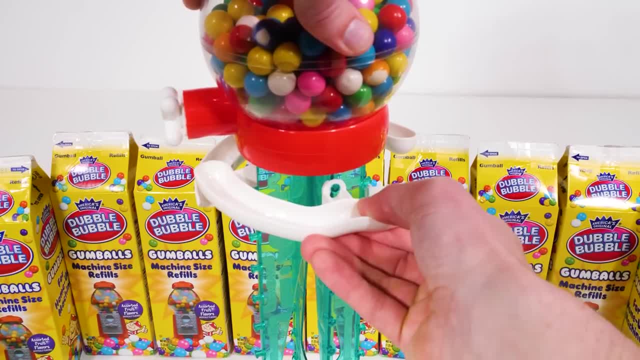 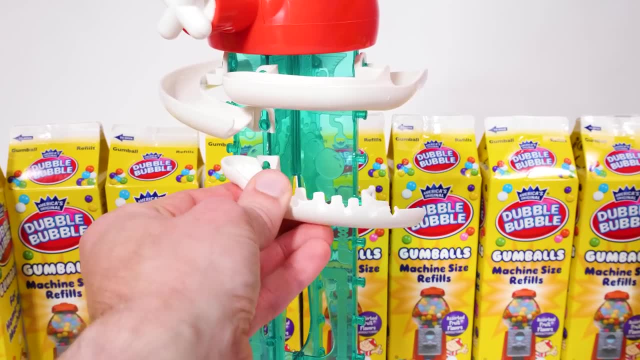 And you can see that this part of the track has bumps that go up and down that'll change the speed of the gumballs as they go down. Next up, we have a new piece. This piece is going to be the holder for our dominoes. 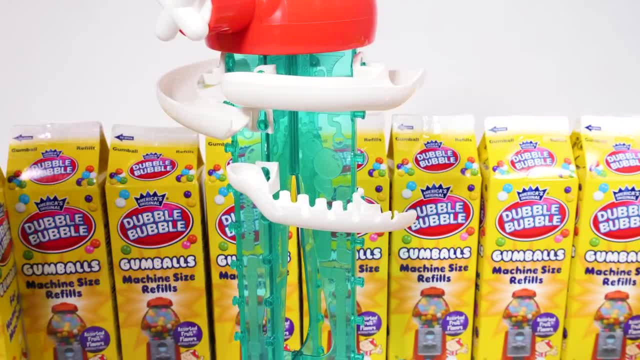 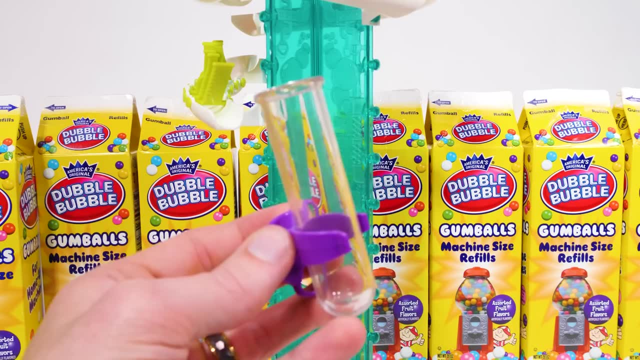 We'll install it on the track first and then we'll add the dominoes to it: One, two, three, four, five, six dominoes. Then we can add our tip over tube, which works kind of like the pendulum. 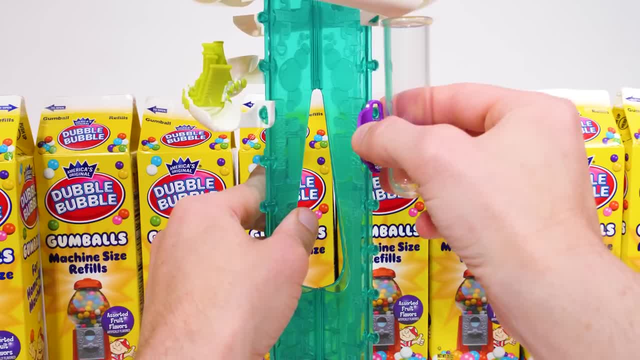 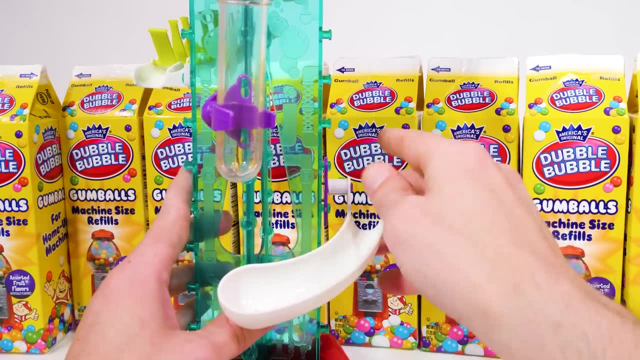 except it doesn't return to a stable state after it tips over Because of its high center of mass. when a gumball falls into it, it'll tip it over and drop it into the track below, So we'll use this piece to catch it. 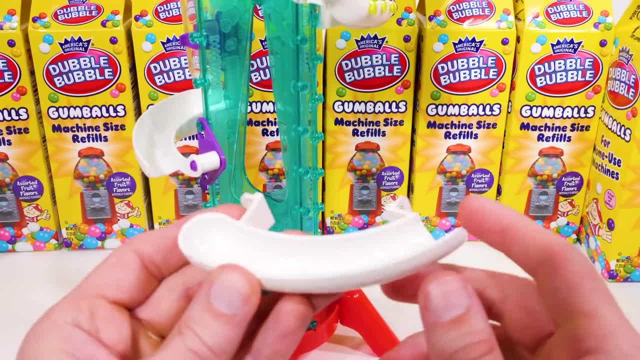 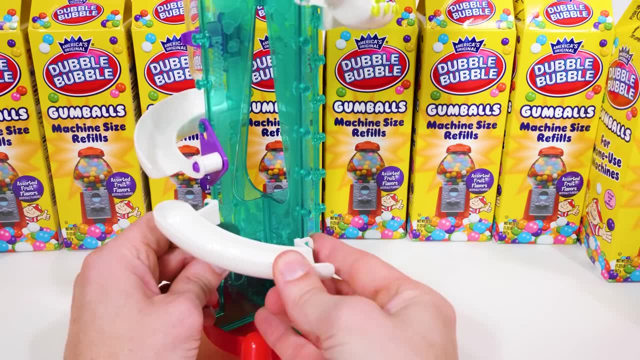 Here's another friction track that uses even bigger bumps to slow the gumballs even more. When they go over these bumps, we might even be able to hear them, And let's just hook it on to make sure it's secure, All right.